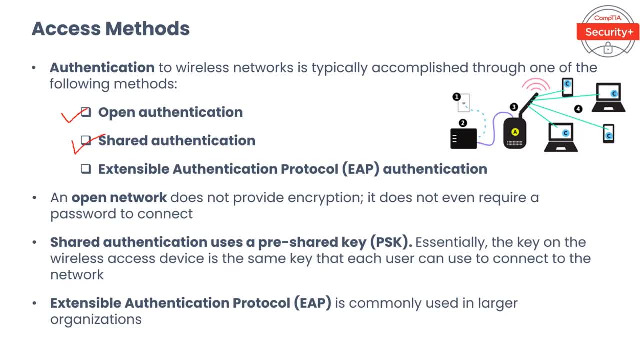 First is authentication: shared authentication and extensible authentication, protocol right or EAP authentication. Although it's not as common as it was once right, the simplest option for many wireless networks is to forego authentication and use an open network. 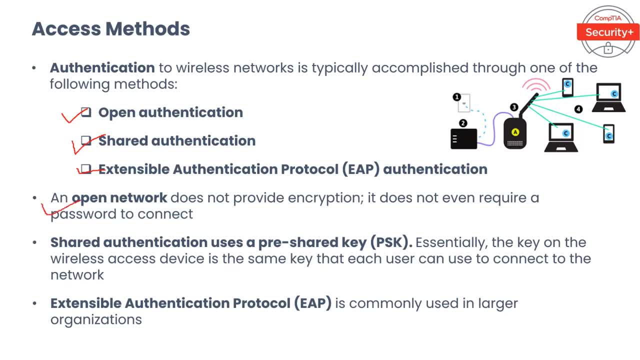 An open network does not provide encryption. It does not even require a password to connect. In fact, an open network does not attempt to provide any security at all. Users simply select the network name or the service, set identifier or SSID for the network. open configuration right for the network. 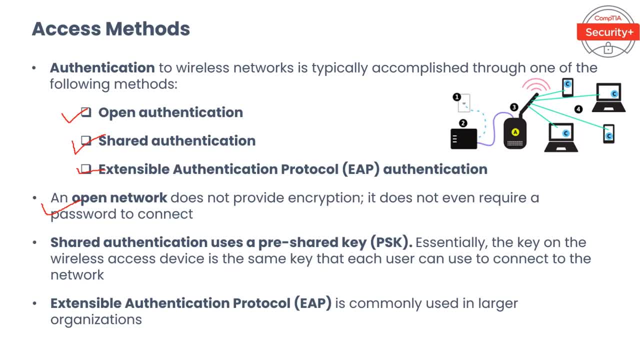 Open configuration is simply not recommended. Some open networks first require the user To connect through a captive portal, which is a web page that is launched first. when connecting through a network, it usually requires some type of interaction before the user is allowed access to other networking or or in it sites. 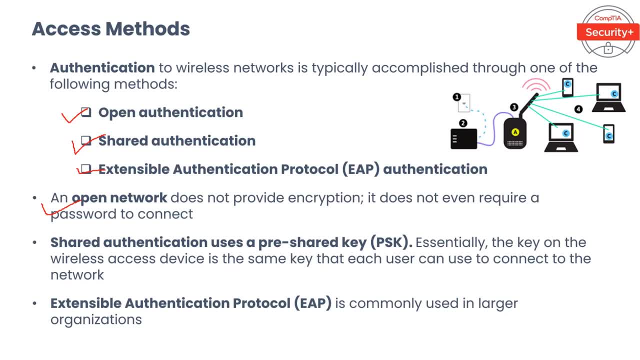 Open networks might use captive portals for advertising or to provide terms of views for the connecting user. Such portals are common in public places such as airports and coffee shops. The user simply clicks Accept views and advertisement provides an email address Right And then. 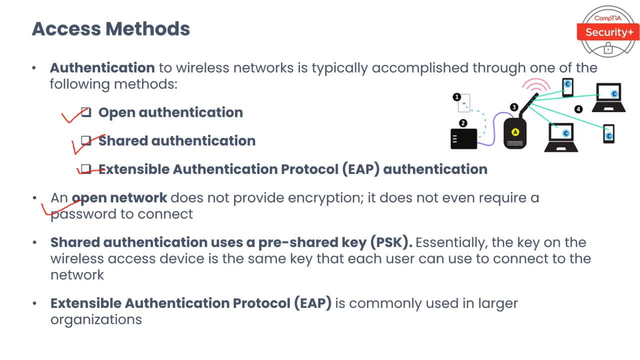 perform some other required action. the network then grants access to the user and no longer holds the user captive to the portal. now the next one is about shared authentication right, which uses a pre-shared key. essentially, the key on the wireless access device is the same key that each user can use to connect to the network. 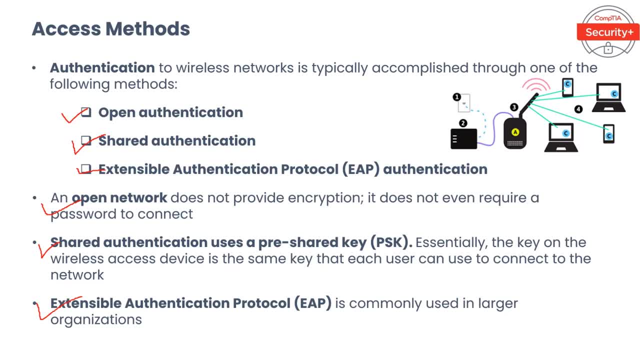 and the third one is the eep protocol, or the extensible authentication protocol. eep is commonly used in larger organization. the authentication process is a bit more involved because an authentication server is required. eep is an extension of point-to-point protocol and allows for flexibility and authentication, including authentication methods beyond just a. 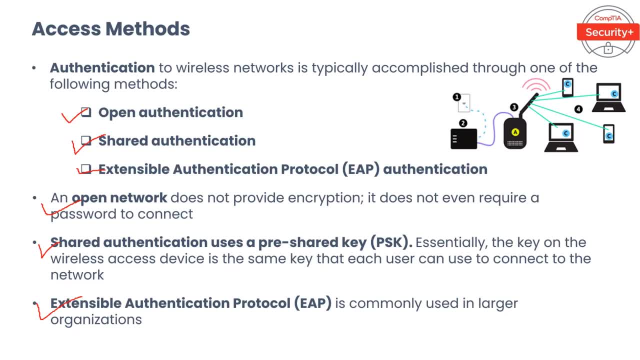 username and password instead of using ppp. however, the ieee 802.1 extender defines using eep over both wired ethernet and wireless networks. eep is a challenge response protocol that can be run over secured transport mechanisms. it is a flexible authentication technology. it can be used with smart cards, one-time passwords and public key encryption. eep. 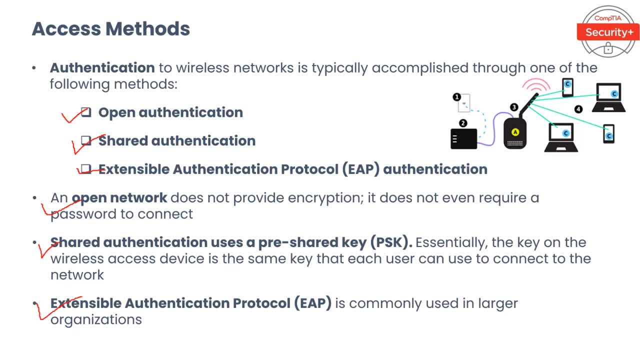 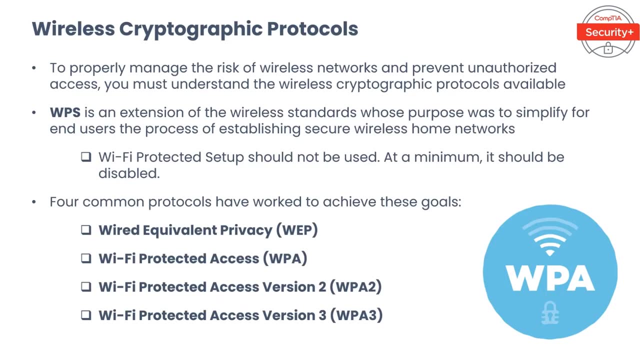 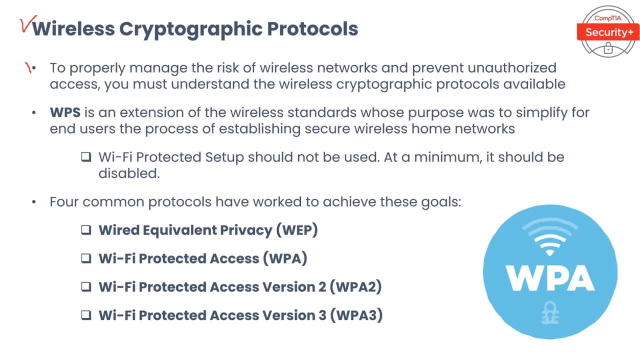 i'll talk about wireless cryptographic protocols. to properly manage the risk of wireless networks and prevent unauthorized access, you must understand the wireless cryptographic protocols available. organizations of all sizes, even home users, need to be aware of the available technologies. the industry has done a lot of help to make technology simple. 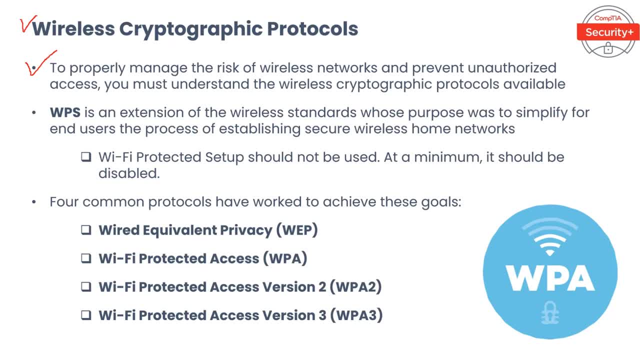 and easy to use, but it has also introduced vulnerable technologies such as eep and eep. it's also introduced vulnerable technologies to make the setup and configuration of wireless clients mindlessly simple. consider, for example, wps or the wi-fi protected setup, originally known as wi-fi um simple config. wps is an extension of the wireless standards whose purpose was to simplify. 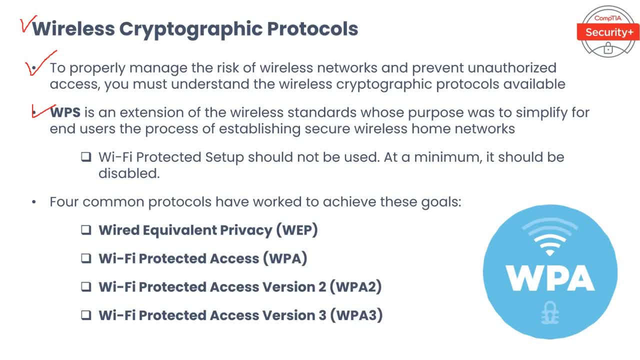 for end users. the process of establishing secure wireless home networks as wi-fi devices and the the mainstream setup was initially complex. consequently, users often run with default configuration, leaving their wireless networks wide open and easy to exploit. so here WPS was introduced as a better option. WPS provides two. 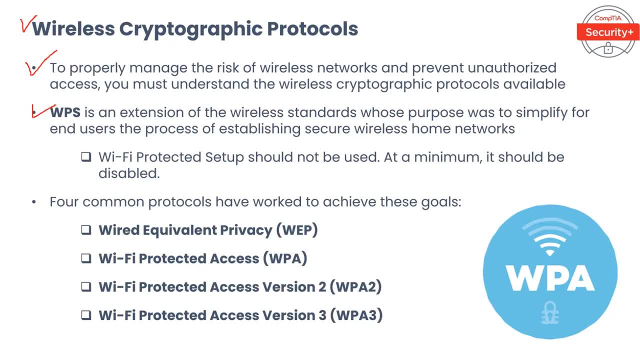 certified modes of operation. the first requires the user to enter a pin code when connecting devices. the second method requires the user to simply push a button on the AP and connect to the wireless device. in 2011, however, a major security vulnerability was exposed. in fact, the vulnerability was so severe. 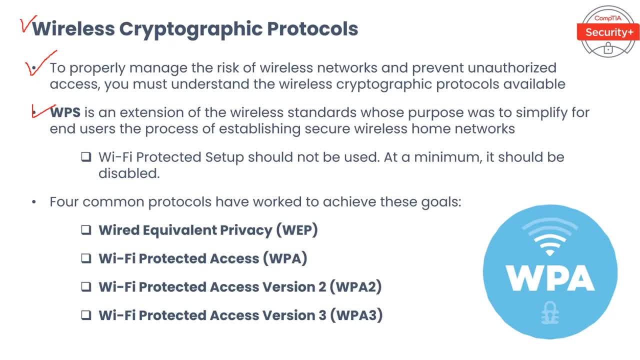 that the solution was to turn off WPS altogether, and it turned out that the user's pin could be recovered through brute force attack in as few as 1100 guesses, or 11,000 guesses, or within several hours in some cases. disabling WPS would cause the user to run out of WPS in a short period of time. 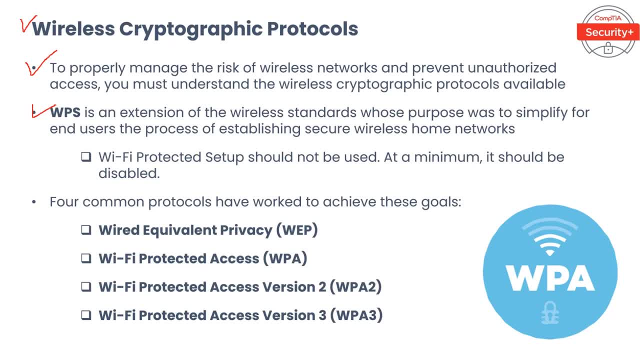 the third installed WPS in玩송 danke was less effective than the first should be, and the third supported Special Temperature assembly. WPS was not even enough to prevent such attacks and a firm or upgrade was required to completely disable the feature. Wi-Fi protective setup raid should. 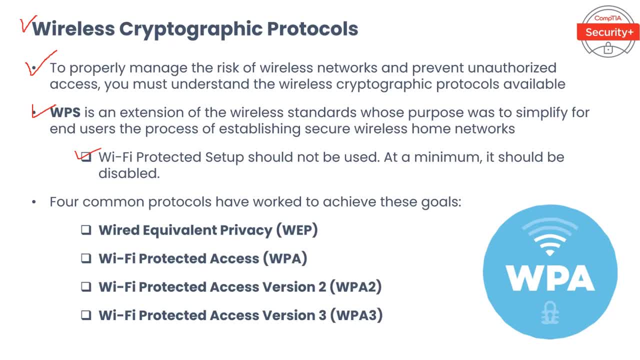 not be used. at a minimum, it should at least be disabled. since WPS was determined to be insecure, several protocols has been developed to protect wireless networks. the primary goals of this cryptographic protocols are tovi sent through the air. there's actually four common protocols that have worked. 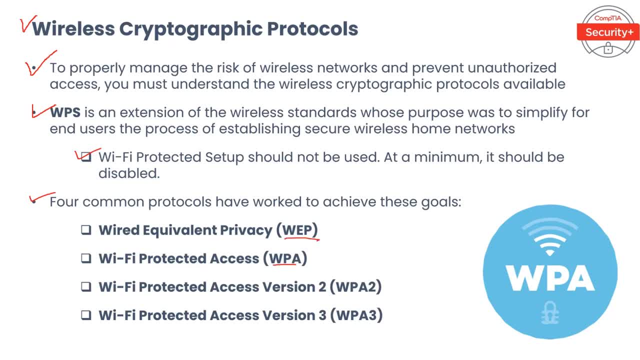 to achieve these goals: the WEPT right, WPA, WPA2 and WPA3. WEPT right or WEP, Wired Equivalent Privacy. this original wireless encryption standard should not be used today, but it is still occasionally is. its goal was to provide security on par with that of wired networks, but WEP has many known security. 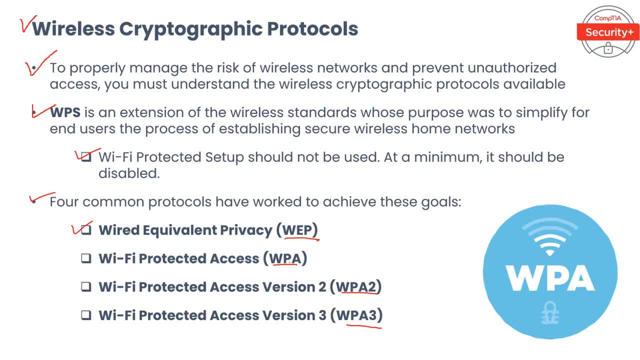 issues, it was superseded in 2003 by WPA. next one is the WPA or Wi-Fi protected access. WPA was developed in response to security concerns over WEPT. WPA is implemented using a couple of different options for encryption, and the third one. 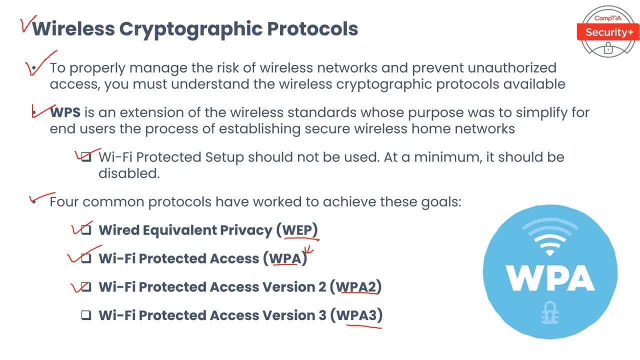 is WPA2. WPA 2 further improved on wpa. since 2006 it has been required for the wi-fi certified devices. wpa2 introduced the use of aes right or advanced encryption standard for encryption, and the third one is wpa3. wpa3 added more features and strengths to the widely adopted wpa2 protocol. 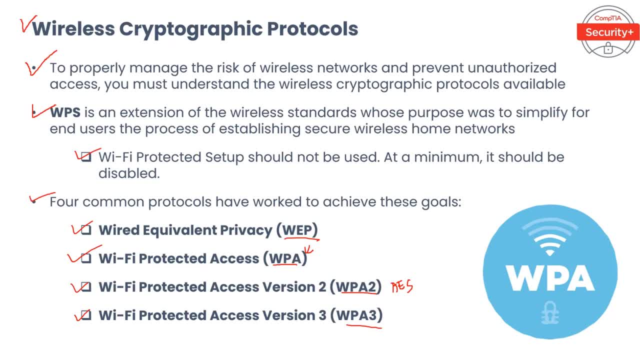 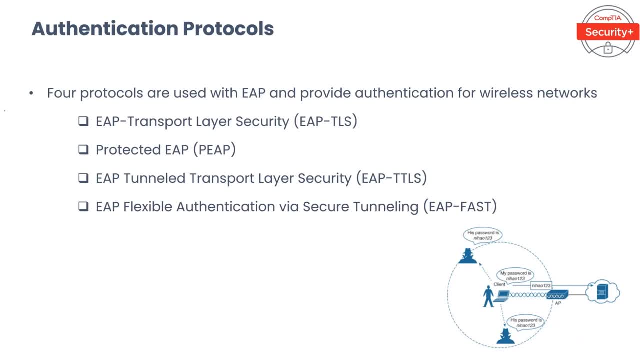 specifically, wpa3 maintains strong cryptographic algorithms while improving the key exchange. let's talk about authentication protocols, exactly four protocols being used with eap and provide authentication for wireless networks. those are eap tls, peep, eap ttls and eap fast. so what are these? let's talk about the first one, which is eap tls. 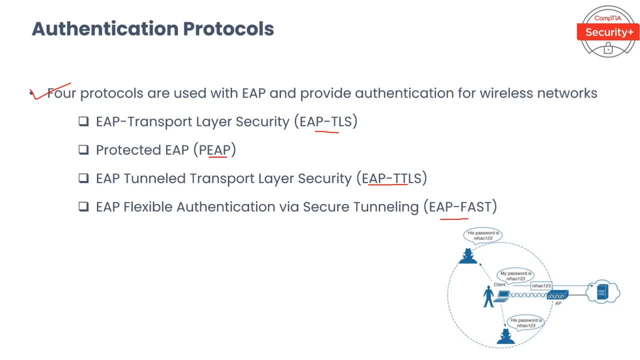 eap tls uses certificate based based mutual authentication, negotiation of the encryption method and encrypted key determination between the client and the authenticating server. EAP messages are encapsulated into 802.1x packets and are marked as EAP over LAN or EAP-ALL. 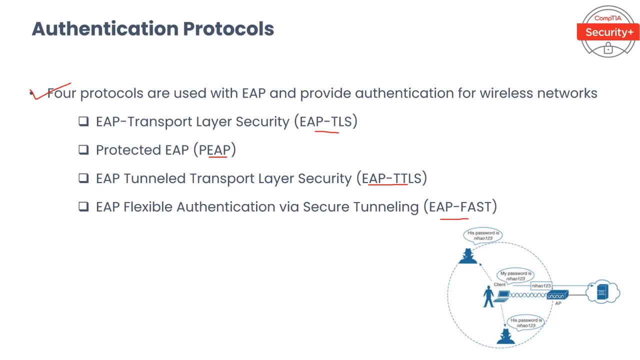 After the client sends a connection request to a wireless access point, the authenticator marks all initial communication with the client as unauthorized. Only EAP-ALL messages are accepted, while in this mode all other types of communication are blocked until credentials are verified with an authentication server. 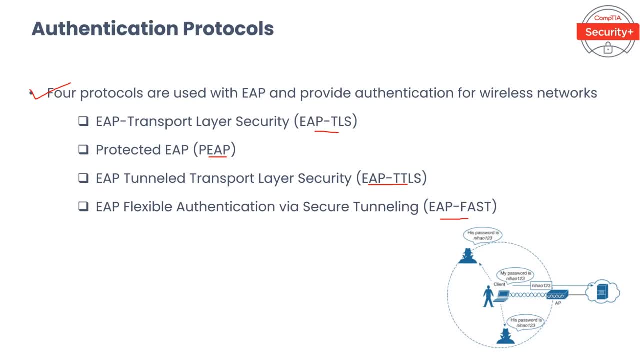 Upon receiving an EAP-ALL request from a client, the wireless access point requests login credentials and passes them to an authentication server. RADIUS is usually employed for authentication purposes. However, 802.1x does not make it mandatory. RADIUS Federation allows a user's valid authentication to be shared across trusted entities. 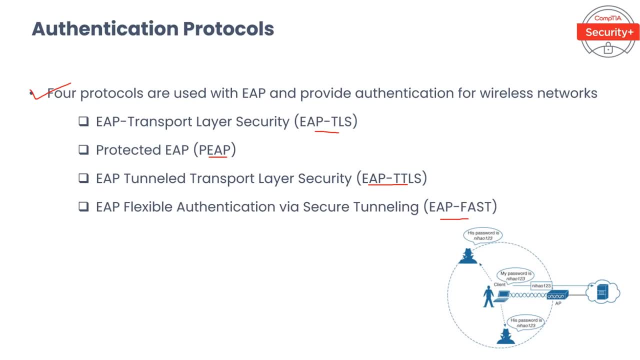 This trust must be established beforehand and the RADIUS server makes assertions about the user's identity and other attributes. This enables users to seamlessly roam across different wireless networks without having to re-authenticate with unique credentials for another entity. Note that RADIUS Federation allows a user's valid authentication to be shared across trusted entities. 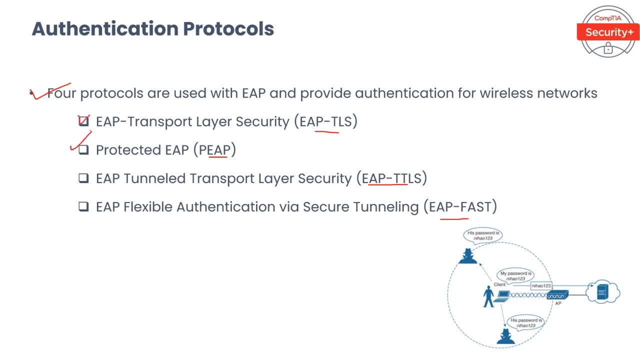 Now let's talk about the next one, which is PEEP, or Protected EAP. PEEP provides several additional benefits over EAP-TLS, including: an encrypted authentication channel, dynamic keying material from TLS. a fast reconnect capability using cached session keys. 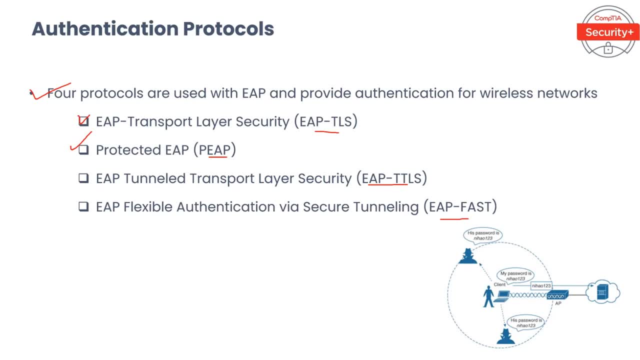 and server authentication that guards against unauthorized access points. PEEP offers a means of protecting another EAP method within a TLS tunnel. PEEP is thus basically a secure wrapper around EAP. It is essentially in preventing attacks on password-based EAP methods. 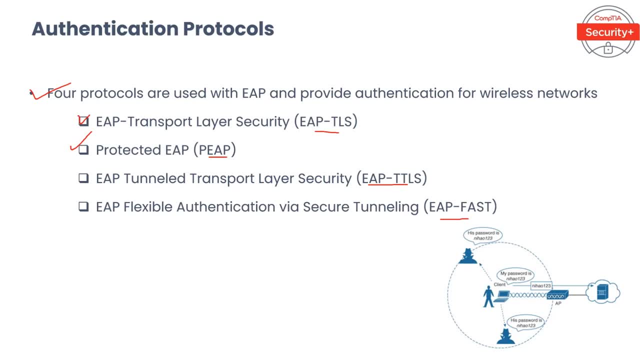 As part of the PEEP negotiation, the client establishes a TLS session with the RADIUS server. Let's talk about the third one, which is EAP-TLS. EAP-TLS is similar to PEEP but further builds on TLS Within an established, secure tunnel. the server authenticates the client using authentication attributes within the TLS wrapper. 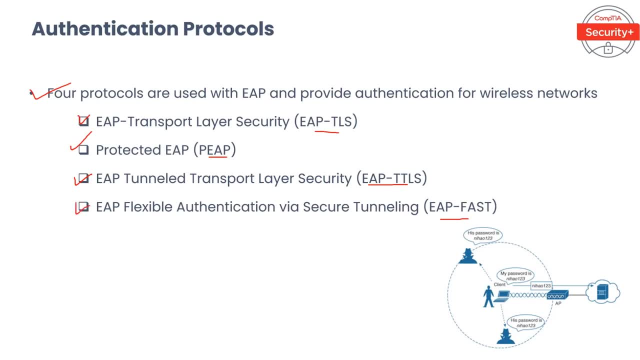 And the fourth one is EAP-FAST, or the EAP- Flexible Authentication via Secure Tunneling. EAP-FAST is a proposed replacement to the Lightweight Extensible Authentication Protocol or LEAP, which for years has been known to contain vulnerabilities. The goal of EAP-FAST is to provide a replacement that is also lightweight but secure. 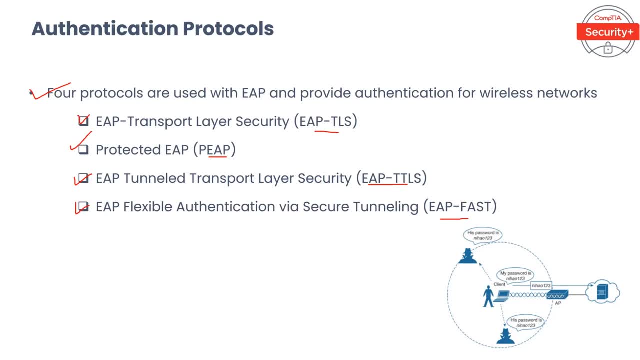 EAP-FAST also works like PEEP, but does not require client or server certificates. Instead, it uses a protected access credential or PACK- okay, let me put it here- which is essentially a shared secret between the client and the server, The client and the authentication server, to establish a tunnel in which authentication is then performed. 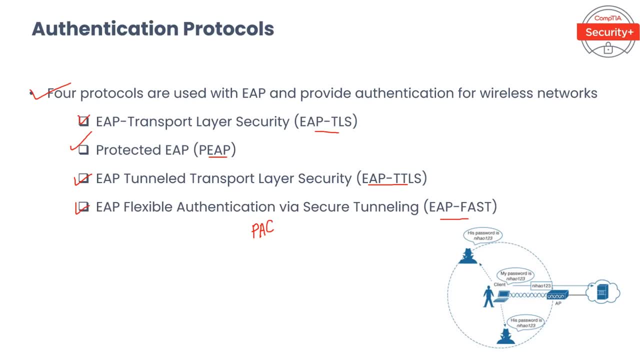 For many organizations that don't want to manage certificates, EAP-FAST might be an ideal alternative to LEAP. Now, each protocol is developed and backed by specific vendors. right, An organization's choice of vendors might dictate the choice of solution. 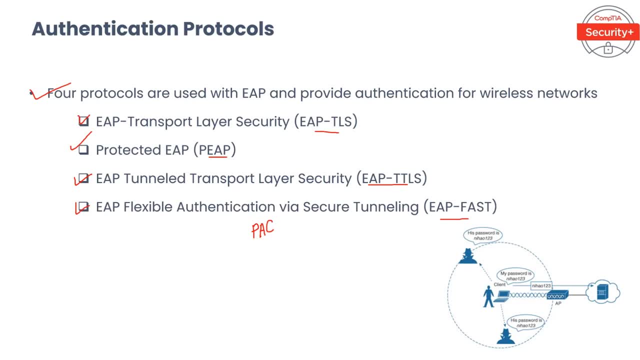 Organizations also need to consider the appetite for managing a certificate infrastructure and deploying certificates not having to worry about certificates, which greatly reduces the burden. for many EAP-TLS requires client and server certificates for mutual authentication. Both PEEP right PEEP and EAP-TTLS eliminate the requirement to deploy client certificate. 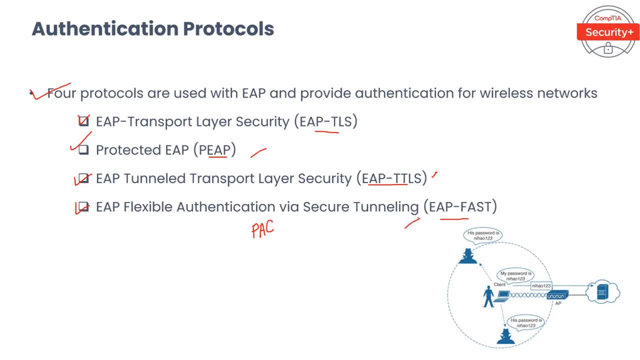 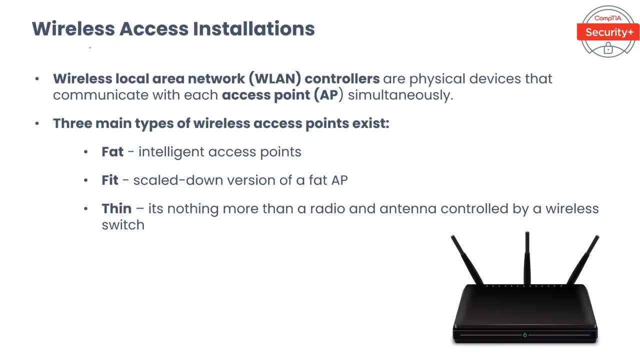 However, EAP-FAST does not require any certificate. Let's talk about the wireless access installation. So no network is complete without a network. Most businesses provide wireless access for both employees, guests and guests. right With this expected convenience, some security implications that must be addressed to keep the network safe from vulnerabilities and attacks. 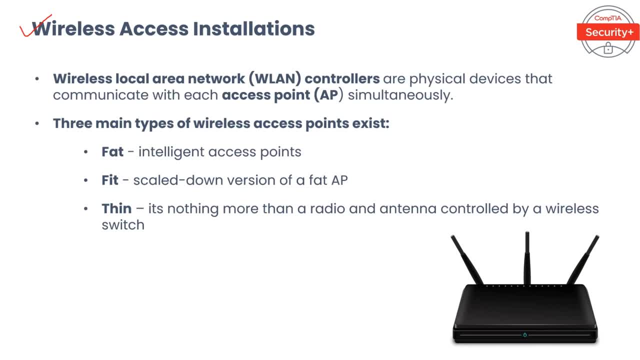 So this lesson covers basic access point types, configuration and preventive measures an organization can implement to mitigate risk and reduce its attack surface. Wireless LAN area network controllers, or WLAN controllers, or WLCs, are physical devices that communicate with each access point simultaneously. 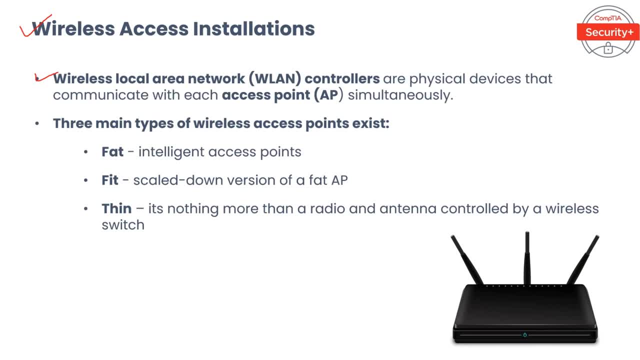 A centralized access controller is capable of providing management, configuration, encryption and policy settings for wireless LAN access points. A controller-based WLAN design acts as a switch for wireless traffic and provides 10 APs with configuration settings. Some ACs or access controllers perform firewall, VPN, IDS, IPS and monitoring functions. 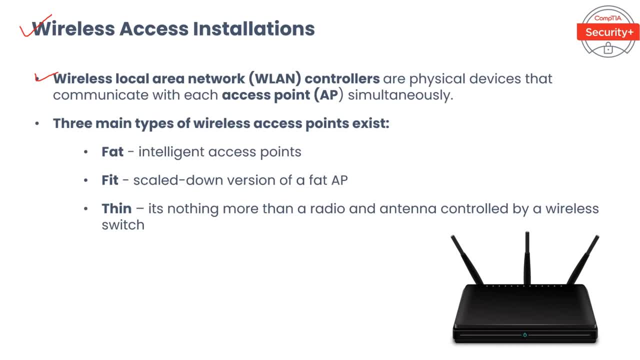 Some ACs or access controllers perform firewall, VPN, IDS, IPS and monitoring functions. The level of control and management options an AC needs to provide depends on the type of access points the organization implements. There are three main types of wireless access points that exist: FAT, FIT and TIN. 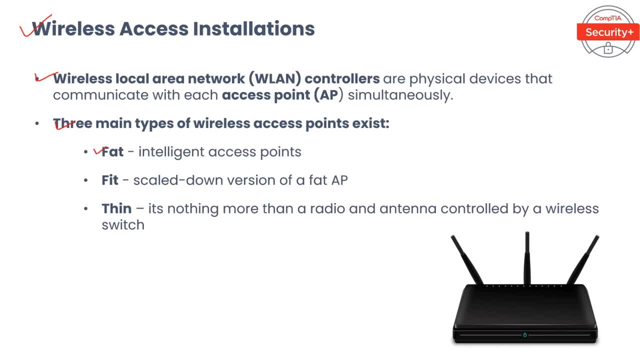 So FAT wireless access points are also sometimes called intelligent access points, because they're all inclusive. They contain everything needed to manage wireless clients, such as ACLs, QoS functions, WLAN support and band steering. FAT APs can be used as standalone access points and do not need an AC. 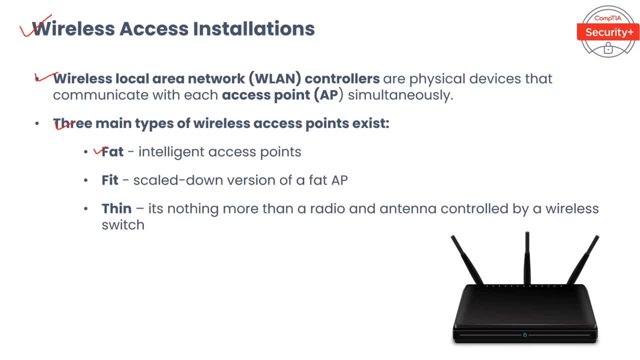 However, this capability makes them expensive because they're built on powerful hardware and require complex software. Next are FIT access points. A FIT AP is a scaled-down version of a FAT AP and uses an access controller for control and management function. The third one is a TIN access point. 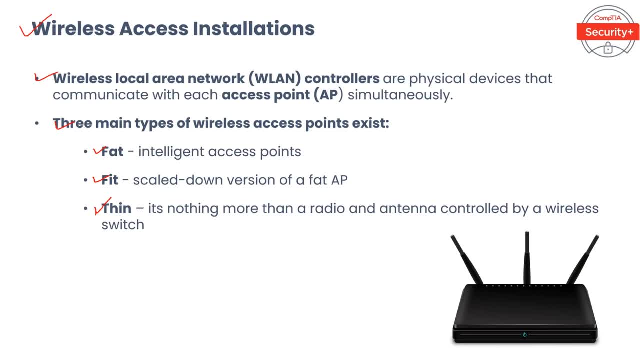 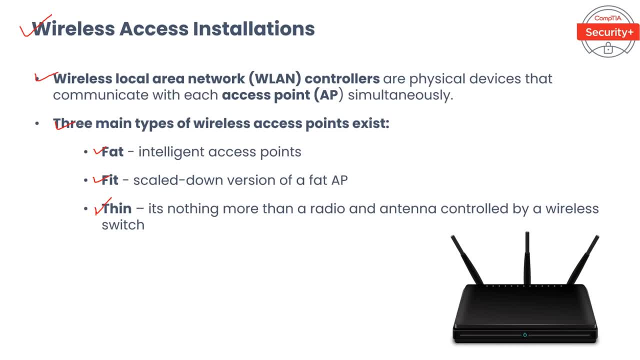 TIN. access points are sometimes called intelligent antennas. In some instances, APs or access points do not perform wireless LAN encryption. They merely transmit or receive their encrypted wireless frames. A TIN AP has minimal functionality and a controller is required. TIN APs are simple and do not require complex hardware or software. 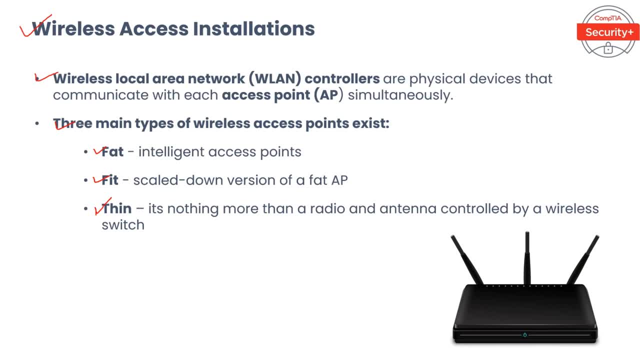 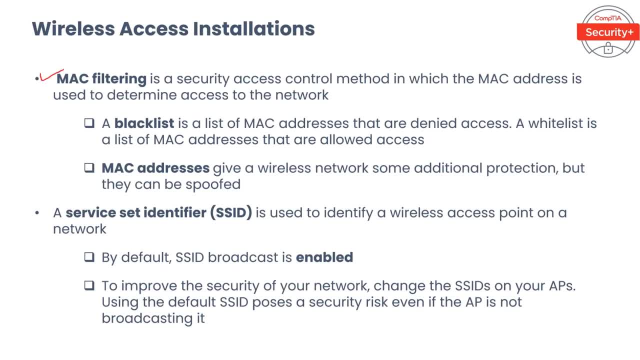 Some additional concepts. Let's talk about MAC filtering. MAC filtering right. most wireless network routers and access points can filter devices based on their MAC addresses. A MAC address is a unique identifier for network adapters. MAC filtering is actually a security access control method. 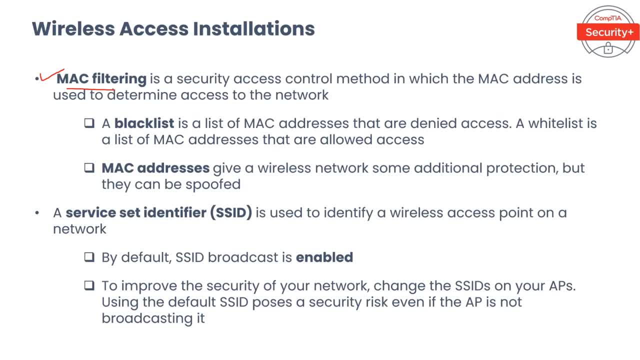 in which the MAC address is used to determine access to the network. When MAC address filtering is used, only the devices with the MAC addresses configured in the wireless router or access point are allowed to access it. So this Ooooh, even though you already have the MAC address. 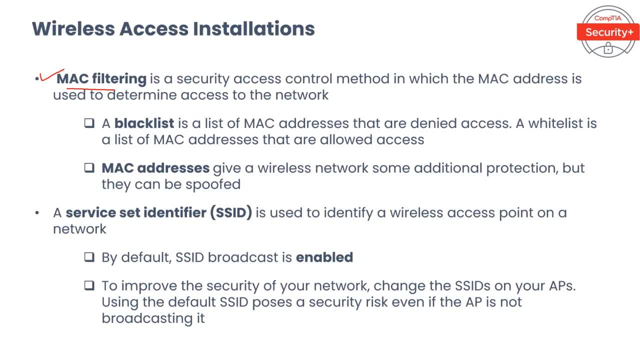 this Oooh, even though you already have the MAC address connect. mac filtering permits and denies network access through the use of blacklist and white lists. a blacklist is a list of mac addresses that are denied. however, a white list is a list of mac addresses that are allowed access. right. so mac addresses gives a wireless network some additional. 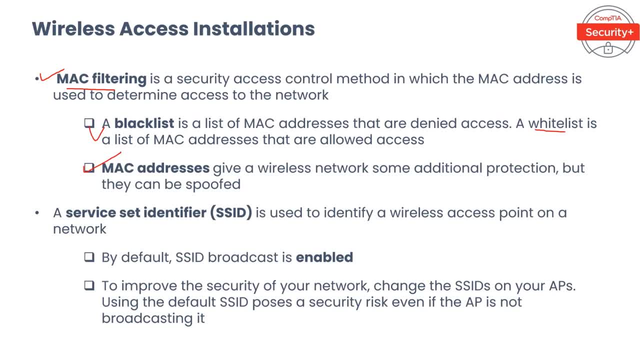 protection, but they can be spoofed. an attacker can potentially capture details about a mac address from the network and pretend to be the device in order to connect to the network. mac filtering can be circumvented by scanning valid mac- uh, valid mac using a tool such as aerodump ng or aircrack. 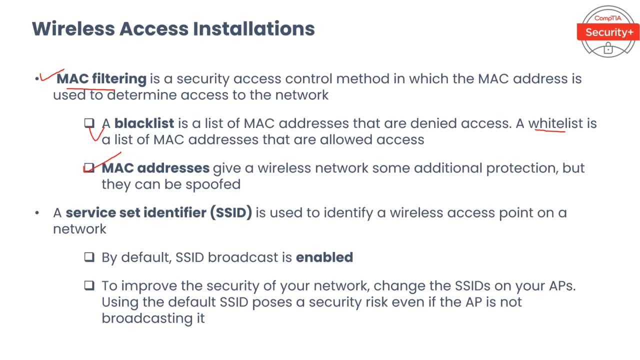 ng suite and then spoofing one's own mac address into a validated mac address. when an attacker knows a mac address that is not in the blacklist or is in the white list, mac filtering is almost useless now. another best practice is disabling ssid broadcast. so note that an ssid or service set identifier is used to identify a wireless access point on 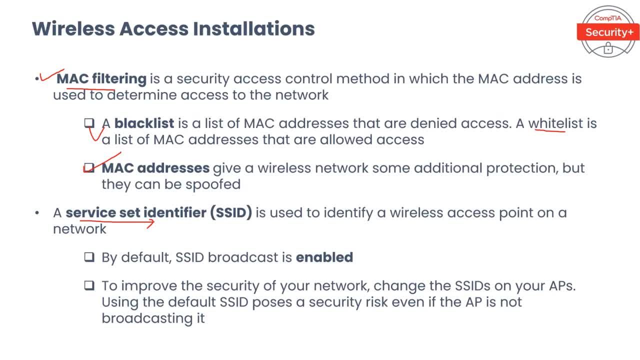 the network. the ssid is transmitted so that wireless station searching for another connection can find it. by default, ssid broadcast is enabled when you disable this feature. that's id configured in the clients must match the ssid of the ap, otherwise the client cannot connect to the ap. having ssid broadcast enabled essentially makes your ap visible to any device through the. 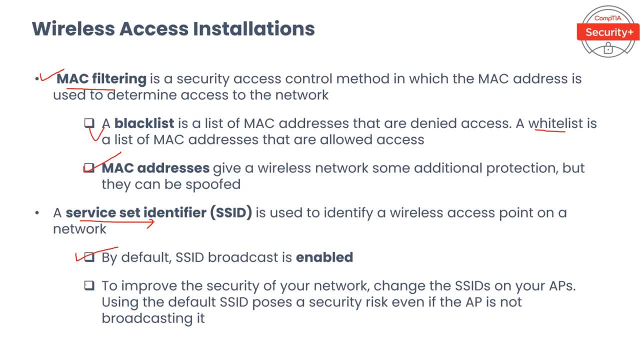 ssid port to access the network. i have a message explaining the ssid port on my cd to the web page to searching for a wireless connection. now, to improve security of your network, change the ssids on your aps. using the default ssid poses a security risk even if the ap is not broadcasting it. 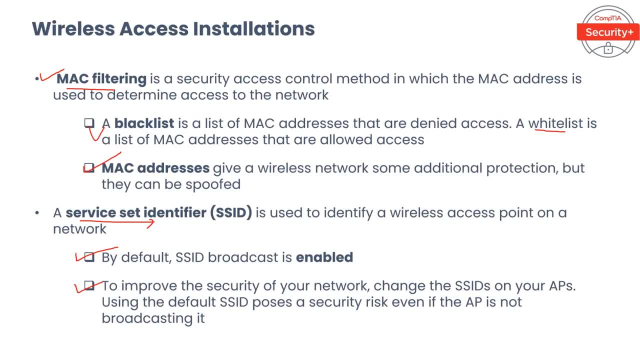 when changing default ssids, do not change them to reflect your company name, main names, divisions, products or address. using such guessable ssids would make you an easy target for attacks such as war driving. we're flying and we're talking with war driving a person in a moving vehicle. 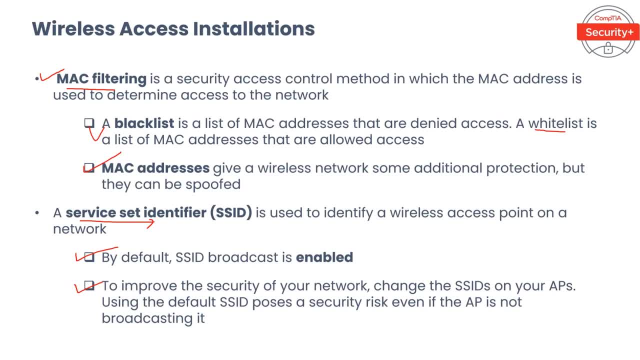 searches for wireless networks using a portable computer or another mobile device. wire flying is similar, but involves the use of aircraft or drone technology. wire wire talking involves drawing symbols in public places to advertise open wi-fi networks. keep in mind that if an sid name is enticing enough, it might attract hackers.